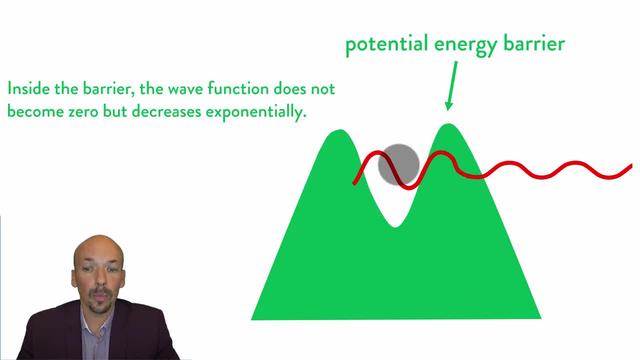 but there's also a small chance to find it here, And in that way this particle can leave the potential energy barriers and go through them and it can come here And it will not cost energy. Only the chance of doing it again will be lower, but it will not cost energy And this can only. 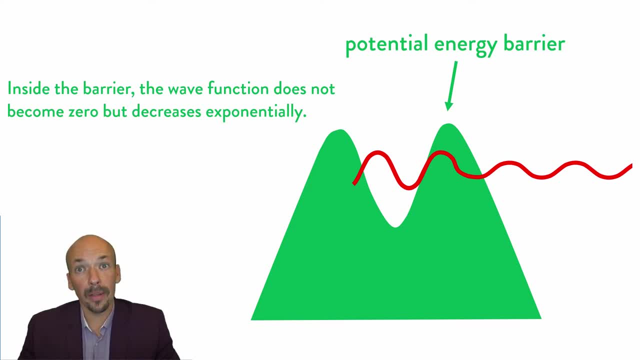 be done by particles which have a wavelength which is around the same magnitude as this potential energy barrier, And this is called quantum tunneling. So this particle in between those potential energy barriers can go through. So how does it work? Quantum particles have a 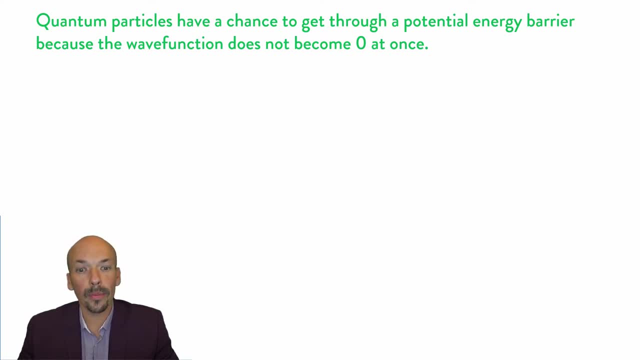 chance of going through a potential energy barrier, because the wave function does not become zero at once. So here you see a wave inside two potential barriers and you can see here that it doesn't become zero at once And here also it doesn't become zero at once. And if this 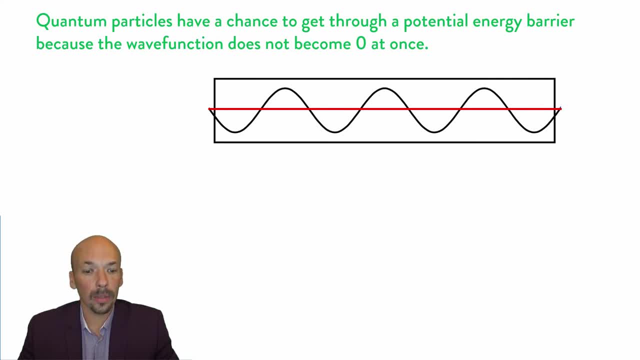 barrier is thin enough, then it will continue on outside of these two energy barriers. This has to do with the de Broglie wavelength, which is this equation- Now you probably know because of my previous video- And also has to do with Heisenberg, which is this equation. So the wavelength 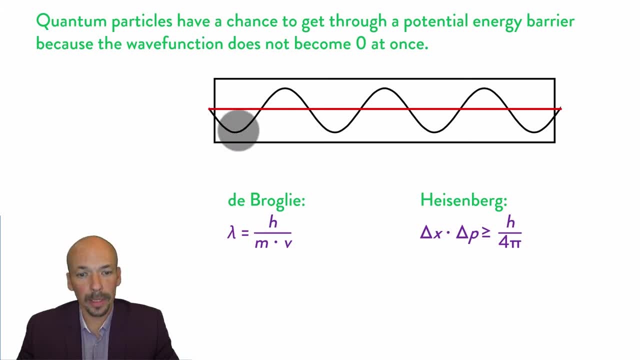 this one says that all particles have a certain wavelength, and that's this wavelength. And Heisenberg says that you cannot for certain know something's velocity when you are certain where that position is, So that way it doesn't become zero at once. So there is a chance to find a. 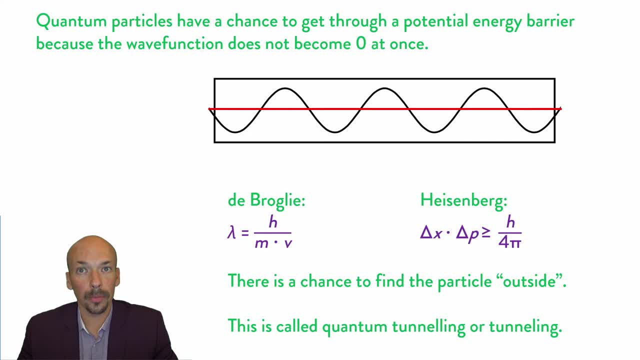 particle outside, And this is called quantum tunneling, or tunneling for short. And this is helping us to understand the quantum world, Because there were certain things we were observing in the quantum world and we could not put our finger on it. why that's the case? And because of quantum. 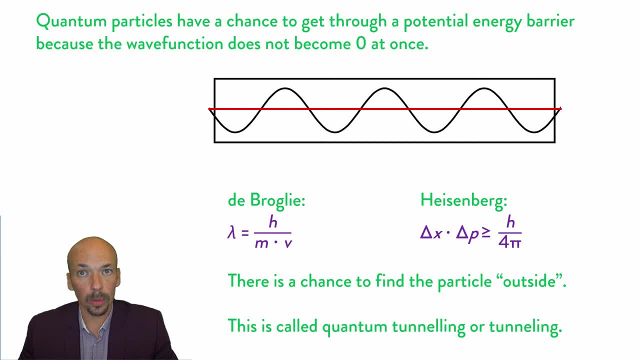 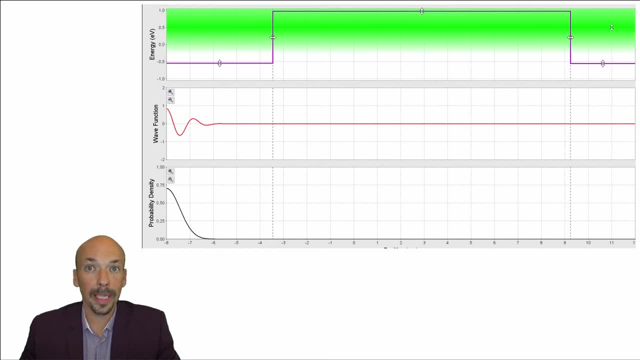 tunneling, we now understand a little bit more about the quantum world and why certain things are happening. So what you will see here is a wave which will be hitting an energy barrier. So here you have the energy barrier And here you have a wave which will go to hit the energy. 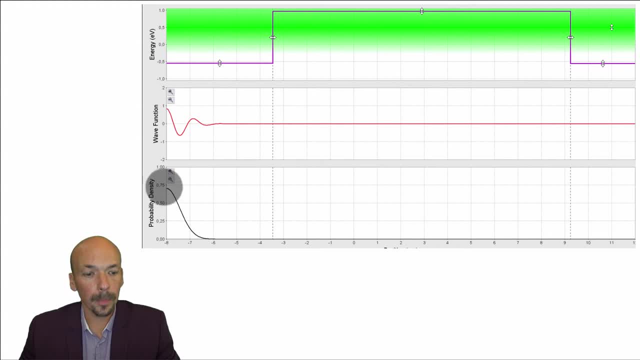 barrier And we will be able to see if it can pass. Here you will see the probability, where you can find the particle. So this is the square of this wave function. So where can you find this particle? Let's see how this goes. So the wave is now going to hit the energy barrier. You can see. 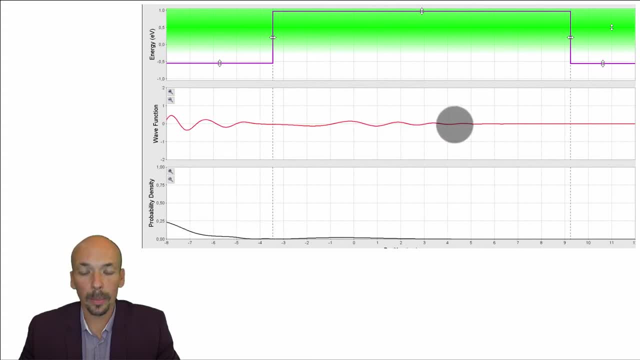 that it doesn't become zero at once And it doesn't become zero at once And it doesn't become zero once. it will go through a little bit and here at the end you will see that it comes out, but the chance of finding it. you can also see it here. it's really 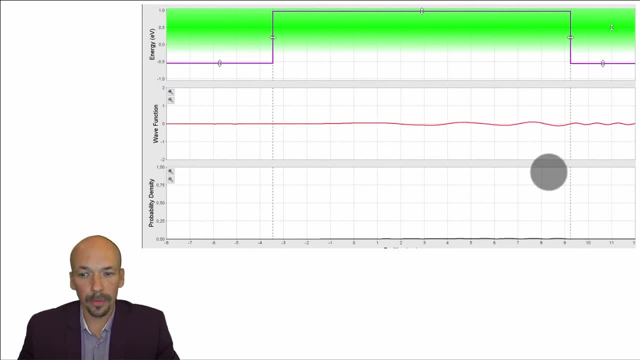 small. so now we're tunneling, you will have a very small chance of finding the particle at the other side. this is because the distance is very large. if you make it smaller like this, then you will see that now there is a larger chance, a bigger chance for a particle to be found here. it's not that big yet and 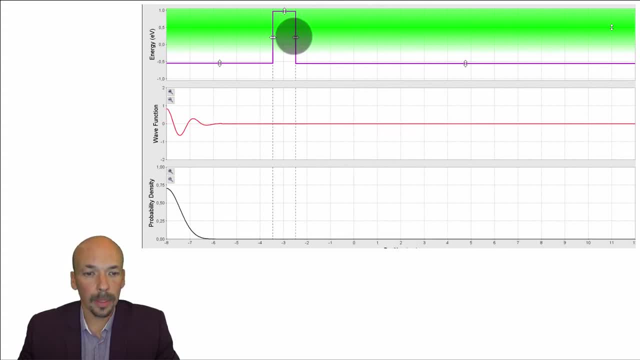 you can also see here a little bit moving. but even if it comes a little bit smaller like this, then you will see that it really will be visible that the particle will be able to be found here. so the wider, not the wider, but the smaller this distance, the bigger the chances that the particle will be found. 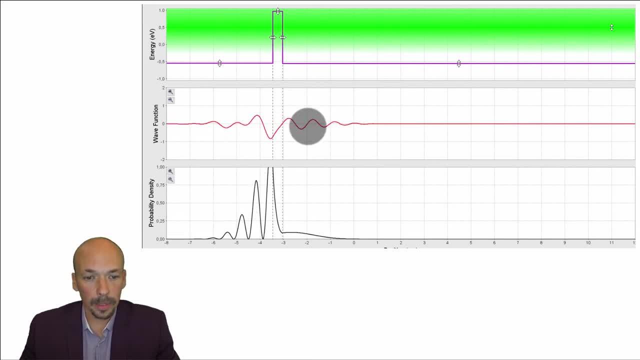 at the other side, and, again very important, this doesn't cost energy. it's just a matter of time of chance. now let's look at the height of the energy barrier. so we now have the starting position and you will see that the particle will have a chance to go. 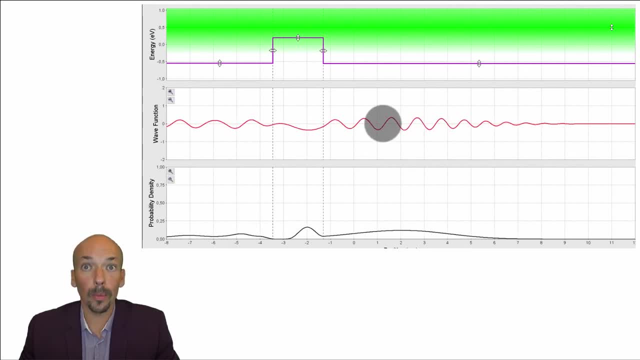 through. so you see here that there is a small chance that the wave will be going through this energy barrier. now, if you make this energy barrier higher, you will see that there are still chance, but the chance will become a lot less. so the higher the energy barrier, the smaller the chances of this particle to tunnel. 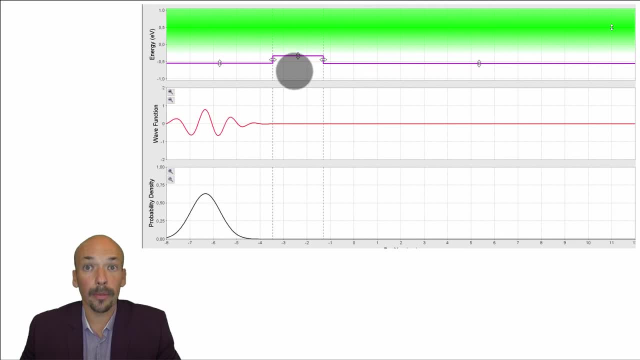 through it other way around. if we make the energy barrier very small, then you can see that the chance of tunneling through this energy energy barrier will also become a larger, because it only is a lot, a little bit of energy it needs to tunnel through. so the 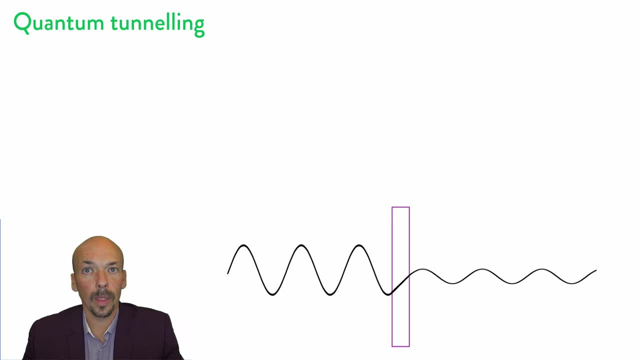 chance will become greater. so in short, a few very important things about quantum tunneling. the de Broglie wavelength needs to be around the same magnitude as the potential energy. then quantum tunneling will take place. quantum tunneling does not cost a lot of energy. quantum tunneling does not cost a lot of energy. 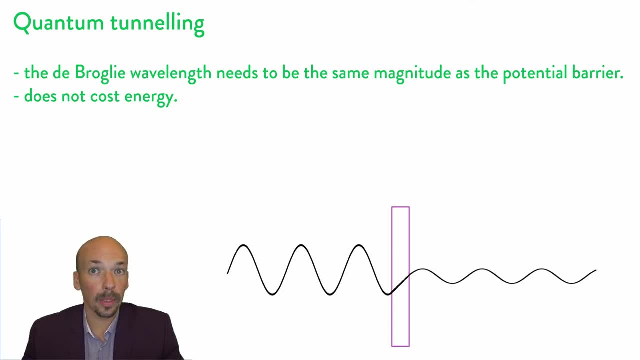 so the particle will be able to pass through a potential energy barrier without losing energy itself. the chance to tunnel again will become smaller. so if a particle tunnels one time, it will have a smaller chance to tunnel again. the probability of tunneling decreases if the barrier becomes taller or wider. 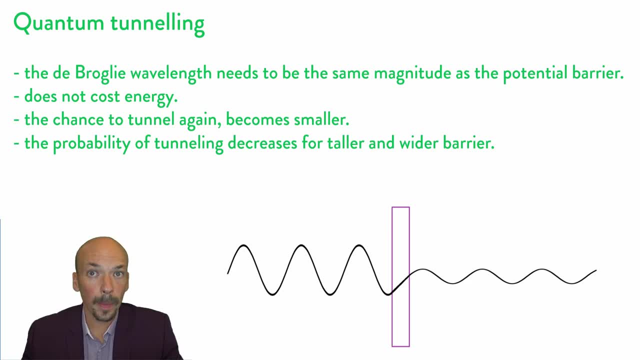 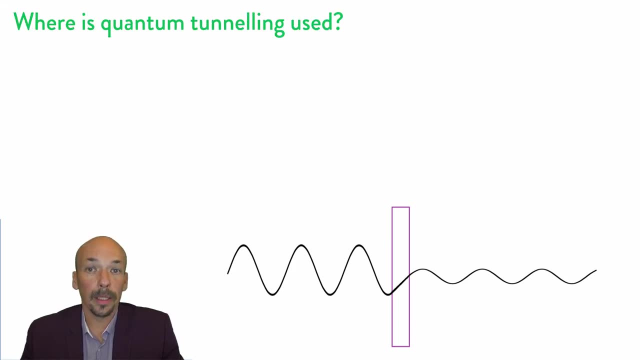 so if it will cost more energy to go through normally, then it will also have a smaller chance to tunnel through it, and also when the barrier becomes wider. so one where is quantum tunneling used? one of the things is radioactive decay, so that's a natural thing with radioactive materials and this is done. 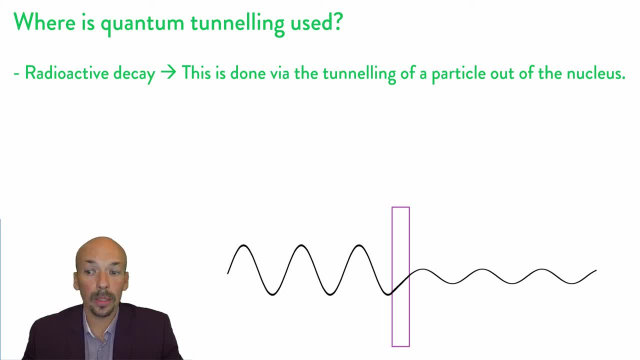 because of tunneling, so the particle tunnels out of the nucleus. normally it would stay into the nucleus and that's pretty tough to get out because there's a lot of energy needed to get out. but it can tunnel out and there's a chance it will do that also. nuclear fusion is possible because the 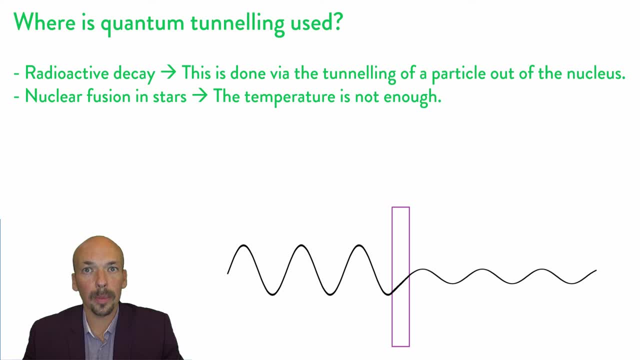 stars, you would think that because the stars are so hot that it happens. but there's even not hot enough to let it happen. so the particles can get very close to each other because of the temperature. and then the last bit is done by quantum tunneling. quantum tunneling is also important for the 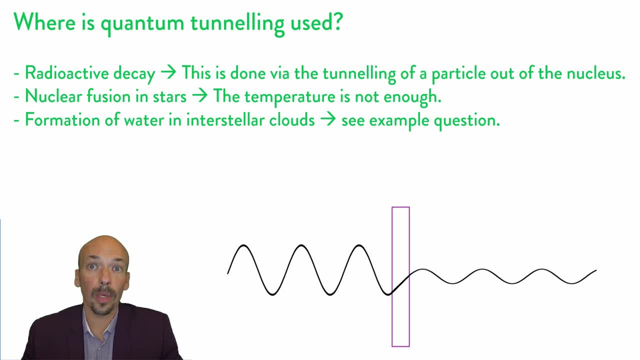 formation of water in interstellar clouds, and I will have an example question which will go more in depth into this. and finally, it's important because it will limit the size of our computer chips. if you will have two electrical wires really close to each other, then there's a chance that the 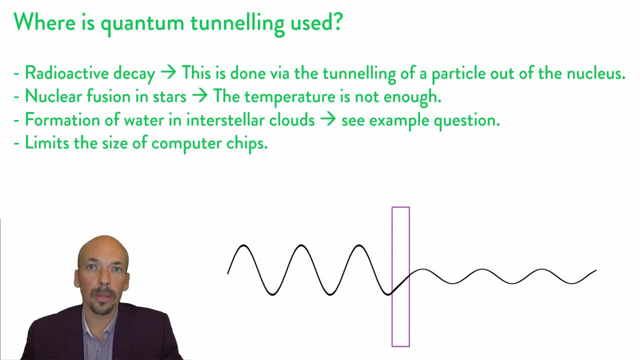 electrons will tunnel between those two wires, and you don't want that in a computer, because then electricity can go wild and then your computer chip will break or it will, it can burn down. so that's why it will limit our computer chips. we cannot make them smaller, because then the electrons inside those 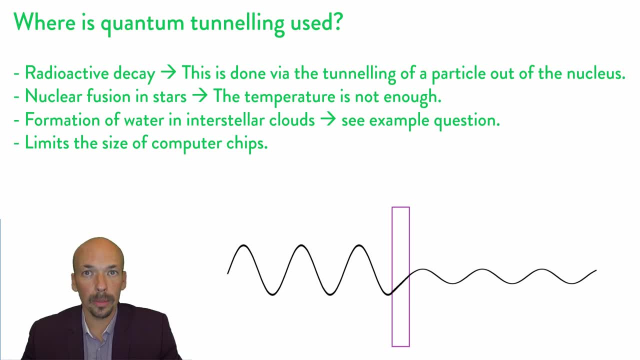 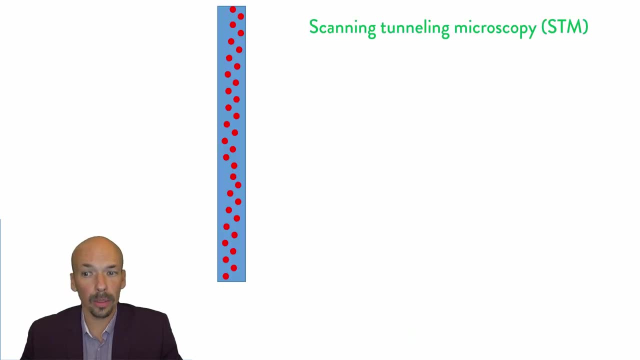 chips. those chips will start to tunnel and there's nothing we can do about that. and one more device where we use quantum tunneling is the scanning tunneling microscope or the STM. and the STM works with a needle- the needle and the material, both have electrons, everything. 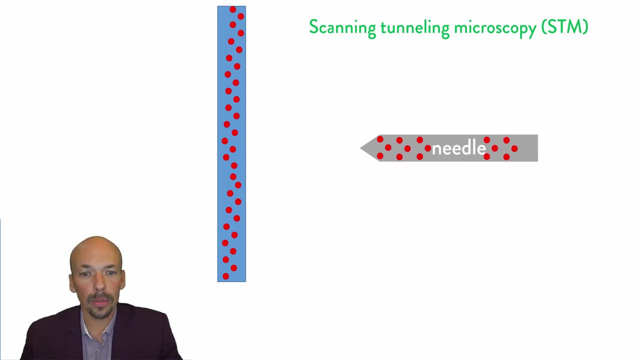 has electrons and the needle will go very, very close to the material, and the moment it's close enough, then of course is happening in a vacuum. then an electron can go tunnel to the needle and this will only happen where they're at a certain distance, so very close, and with this you can go with the needle. 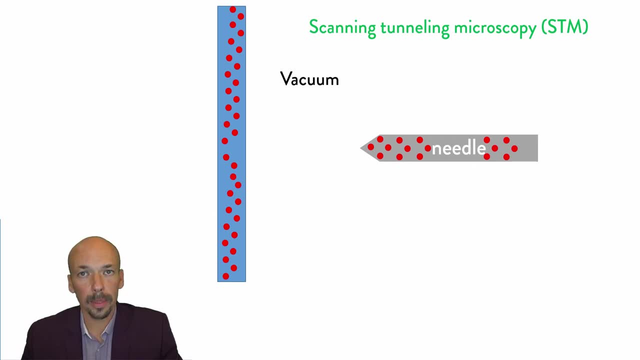 passing the material, and every time an electron tunnels, you know that there is a material. you can get very detailed pictures from this material, so you can scan this and you can actually see molecules by this, and this is called a scanning tunneling microscope and it makes use of the fact that electrons can 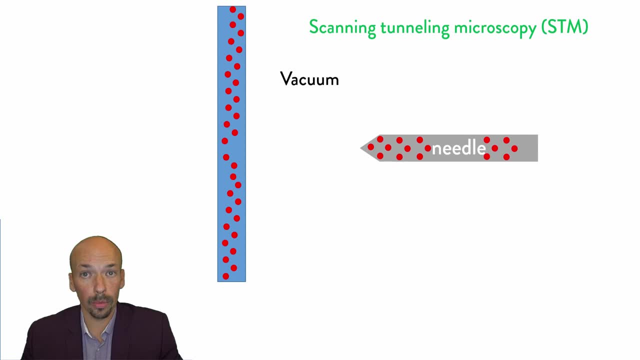 tunnel through a vacuum, because normally the electrons could not go through a vacuum, but with quantum tending they can go through. there will now be three example questions to give you an idea what you can expect with quantum tending, quantum tunneling, in your exam or in your test. 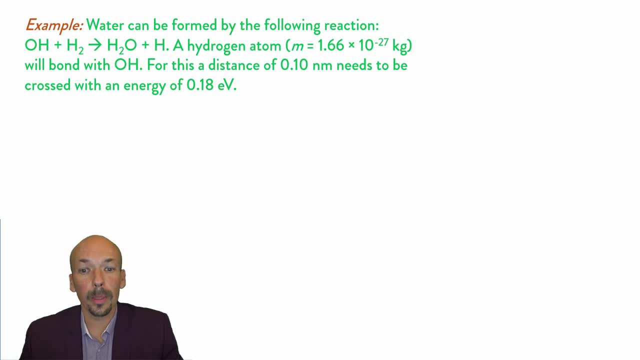 So the first example, water, can be formed by following this reaction, OH plus H2 becomes water. H2O plus H. A hydrogen atom with a certain mass will bond with the OH. For this, a distance of 0.10 nm needs to be crossed with an energy of 0.18 eV. so it looks. 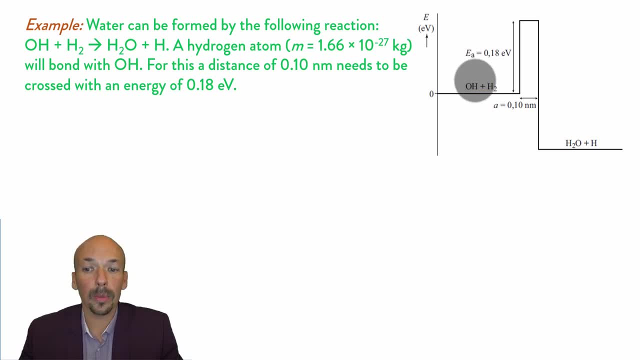 like this. So here you have this H, which will have to jump there, and to do that it needs to either go over this energy barrier- so you need an energy of 0.18 eV- or it can tunnel through, and then it needs to cross this distance. 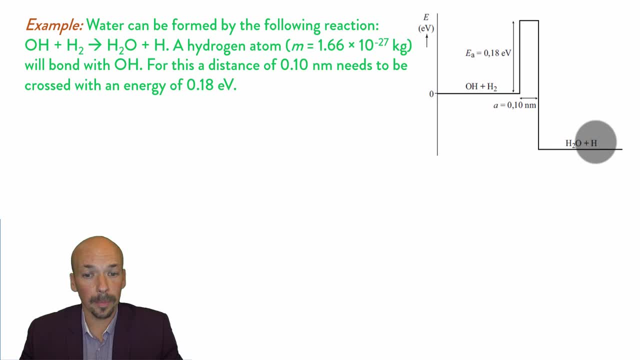 And then it will become here the water plus the H. So you can either get this energy or you can tunnel through, and we will be looking at the tunneling through, how that will work. So we will calculate the velocity of this particle, of this hydrogen particle, when 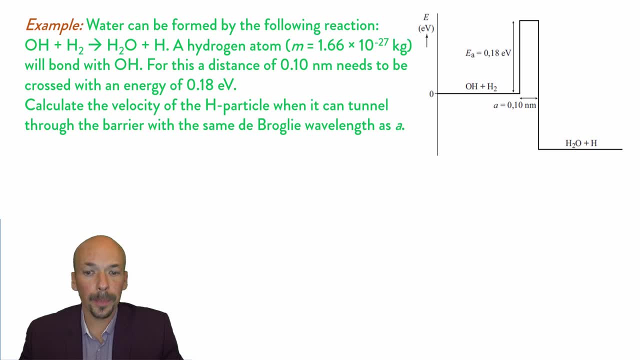 it can tunnel through the barrier, and it will tunnel through when the de Broglie wavelength of this particle is the same as this distance. So we need to calculate the de Broglie wavelength. So try this for yourself by pausing the video now, and I will give the explanation. 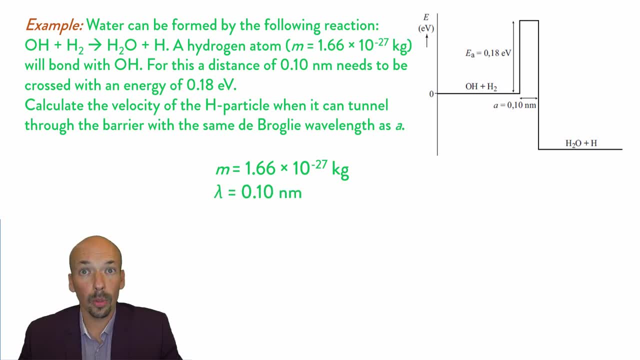 First, we have the mass of the particle. we have the de Broglie wavelength, because it has to be the same magnitude as the barrier itself. We have the Planck constant, which will be needed, and we need to convert this one to: 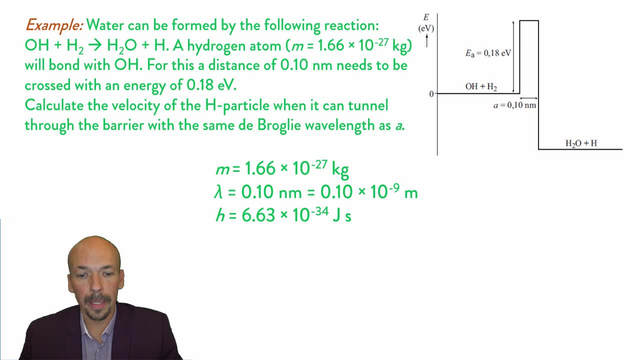 meters. so we divide it by 10 to the power of 9.. And we will use this equation. So the de Broglie wavelength equals the Planck constant divided by the mass multiplied by the velocity. We need to convert this one because we need to actually calculate the velocity. 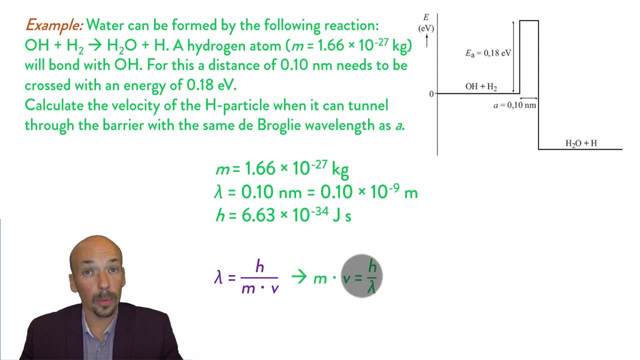 So we can convert by this, we can switch these two. so it will look like this: And now we divide by the mass and it will look like this: This will be the equation we use. We use our information in this equation and we calculate that the velocity needs to be. 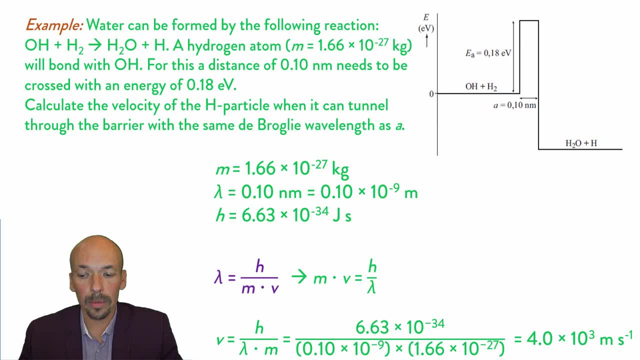 at least, or it needs to be 4.0 times 10 to the third meters per second. And the interesting thing is, this is not the minimum velocity you need. this is the maximum velocity Because if you look at this equation, 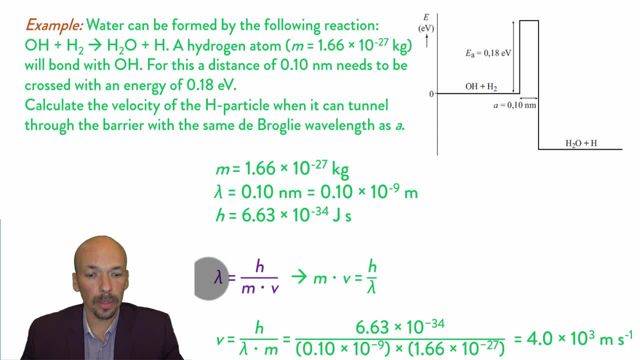 This is the maximum velocity, This one and the de Broglie wavelength. it can be larger. If the de Broglie wavelength will be larger, that's fine, because this one will only be easier to tunnel through. So if this one goes up, that's fine, but it cannot become lower. 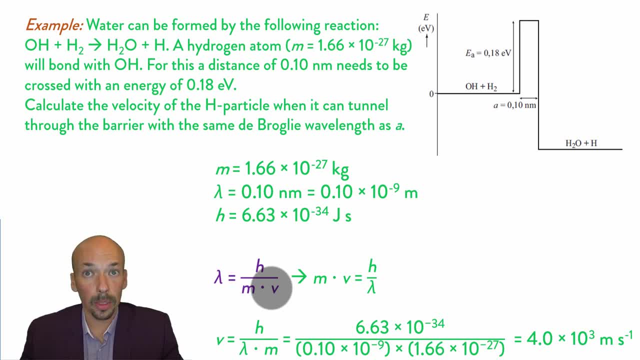 So if this velocity will become higher, so if the particle will start moving a lot faster, then this one will become larger and because it's down here in this equation, it will become a smaller number. so the de Broglie wavelength will become smaller, so it will be harder. 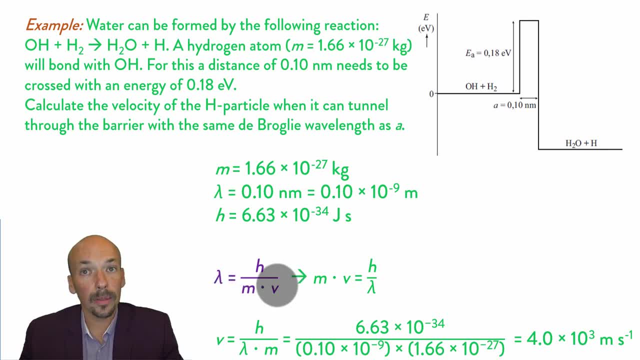 to tunnel. It will not be as easy to tunnel when the velocity goes up. When the velocity will go down, this number will become larger and then the de Broglie wavelength will become larger and it will become easier to tunnel through. 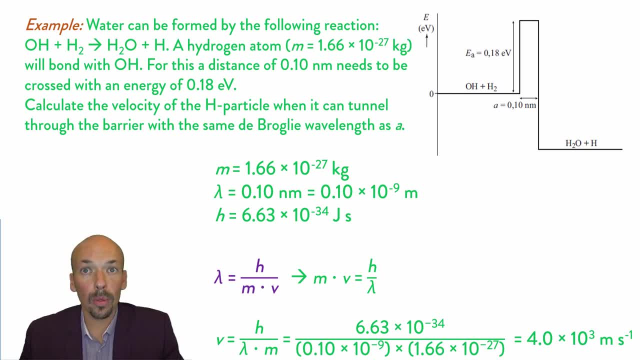 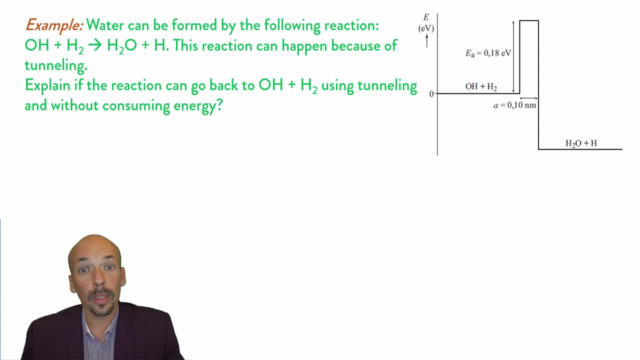 So that's a little bit counter-instinctive. you need a small velocity and then the tunneling will become easier. We will now go to the next example question. So water can be formed by that equation. and now the question is: explain if the reaction 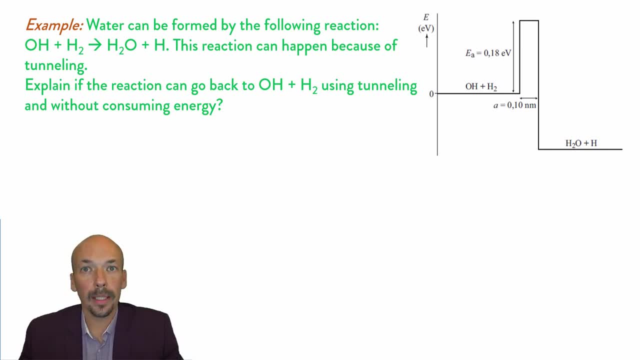 is that the particle can go back to OH and H2 using tunneling and without consuming energy. So this particle tunneled here and we are now here and now the question is: can we go back there with tunneling, but without extra energy? 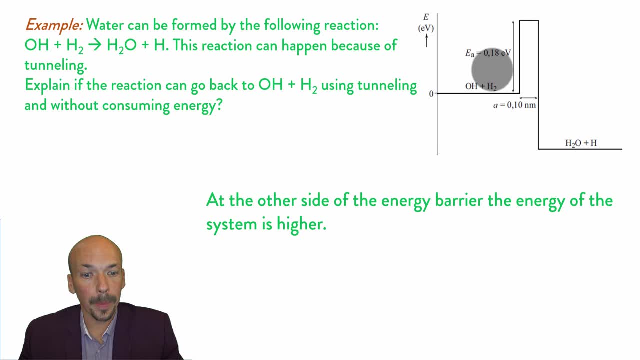 So what do you think? Can this one go tunnel back there? Well, the answer is at the other side of the energy barrier. so here the energy of the system is higher, so this energy here is higher than here, so therefore the particle. 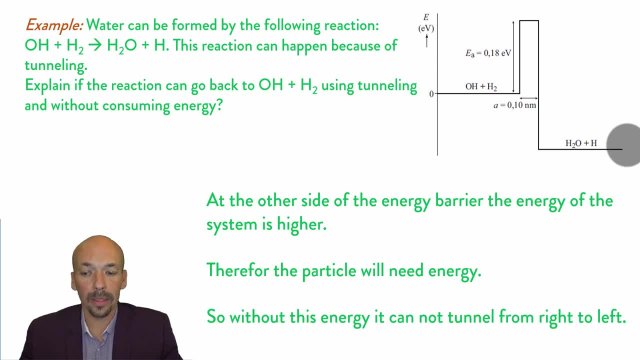 will need energy. So without this energy it cannot tunnel from right to left. So if these energy barriers would be at the same height then, yes, it could tunnel back. But if it now tunnels back it will be here and it will not have enough energy to be here. 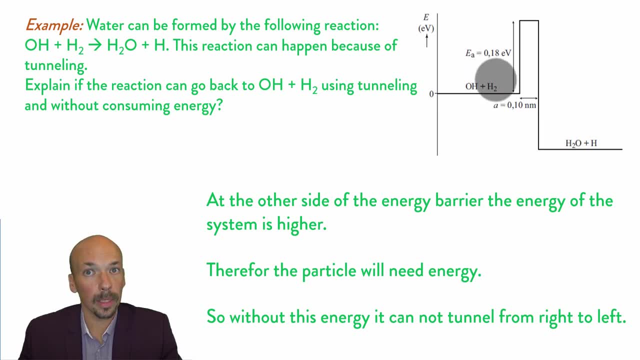 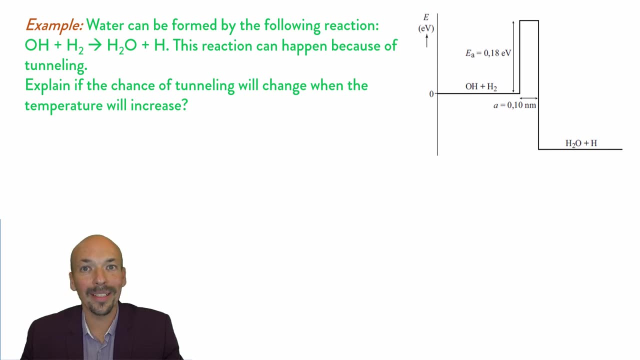 So it can tunnel to here, but then it also needs energy to come here, So without that energy it cannot tunnel back. And now the last example question: explain if the chance of tunneling will change when the temperature will increase. So what will happen when the temperature will increase? 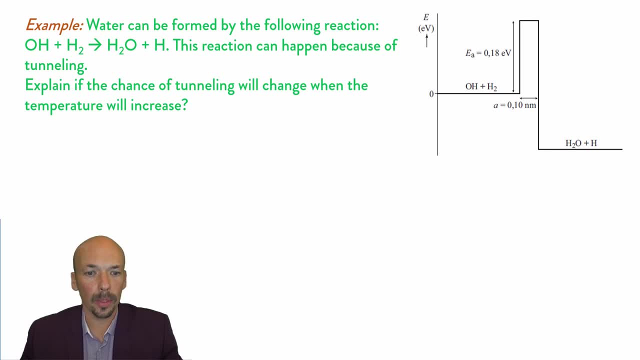 What will happen with the chance of tunneling? Try this for yourself. I will now give the answer. and it has to do with this equation. Just like I said before, it has to do with the velocity. So if the temperature increases, the velocity of the particle will increase. so this one. 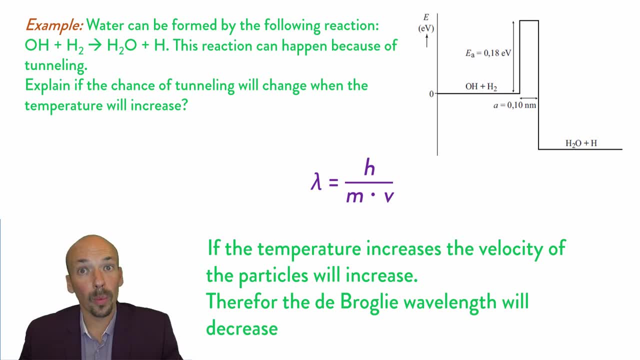 will increase. Therefore the de Broglie wavelength will decrease and the chance of tunneling will also decrease. So the warmer this one will be, the harder it will be to tunnel back. So this one actually works best when it is cold. 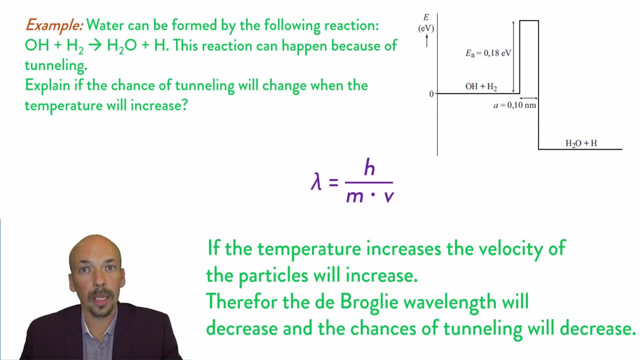 This is also happening at this moment in interstellar clouds far, far away. It is very cold and water is formed by this equation. So with this equation, because of tunneling, water can be formed without using this energy. So, without this energy, water can still be formed. 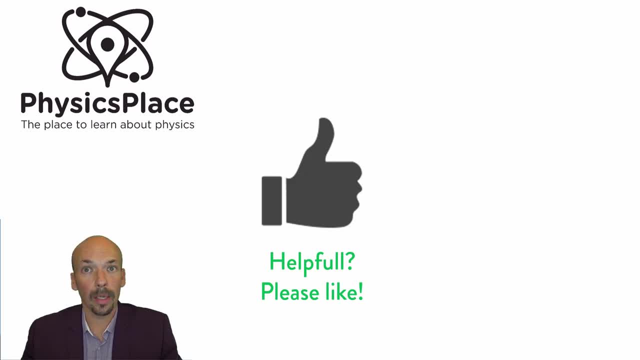 That's it. If you found this video helpful, please let me know by liking And, of course, subscribe. Thanks for watching.